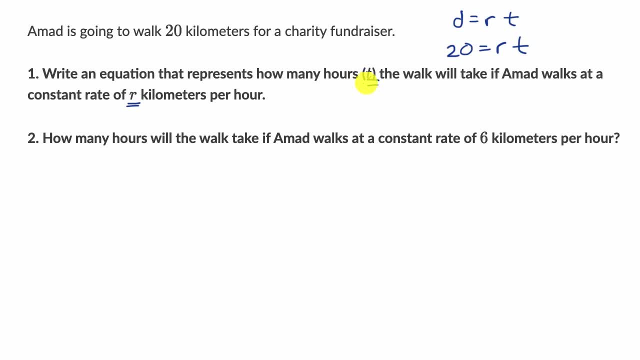 Now they're asking us for an equation that represents how many hours the walk will take if Ahmad walks at a constant rate of R. So, the way that it's phrased, it sounds like they want us to solve for T, where T is going to be equal to some expression here. 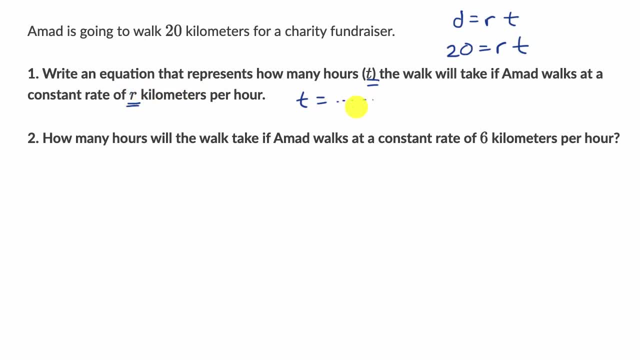 that deals with R and probably some other things. So if we put in any R here then we can get the time. So if we know what the rate is, if you put that in here because it's already solved for T, we'll be able to solve for that time. 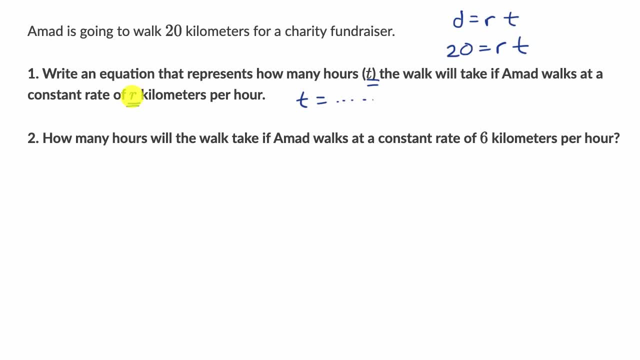 You could think of R as the independent variable, that you could try different values out for, and that T is the dependent variable. It's the thing that we have solved for. So let's do that, Let's rewrite this expression here, by solving for T. 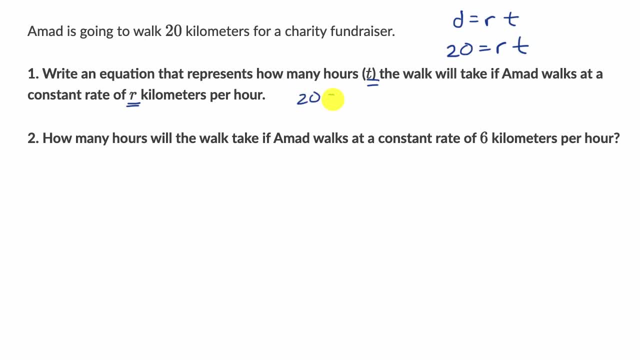 And I could do it right over here. If I have, 20 is equal to RT. if I want to solve for T, what can I do? Well, I could do this. I could divide both sides by R. If I do that on the right-hand side, 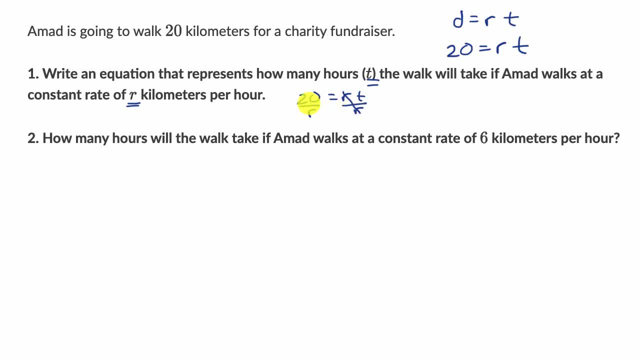 then I'm just left with a T here, because an R divided by R is just one, And on the left I have 20 over R, So I have T is equal to 20 over R And we're done. This will tell us how many hours Ahmad will take to walk. 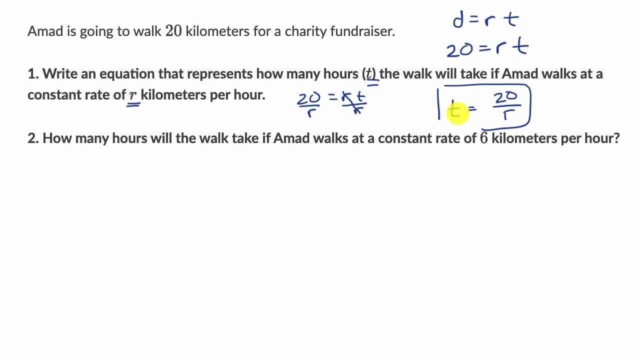 based on the rate. You give me a rate. I'm just gonna divide 20 by that and I'm going to give you T. You might say: why is this useful? Well, this is useful because, now that we have it written this way, 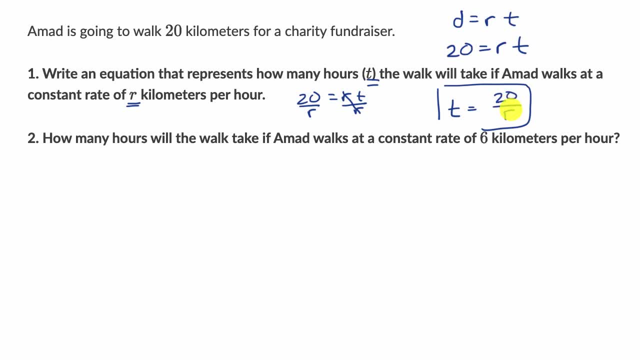 anytime someone gives an R to you, you just take 20 divided by that and it essentially is already gonna solve for what your time is, how far, how long Ahmad's gonna have to walk? Question two: how many hours will the walk take? 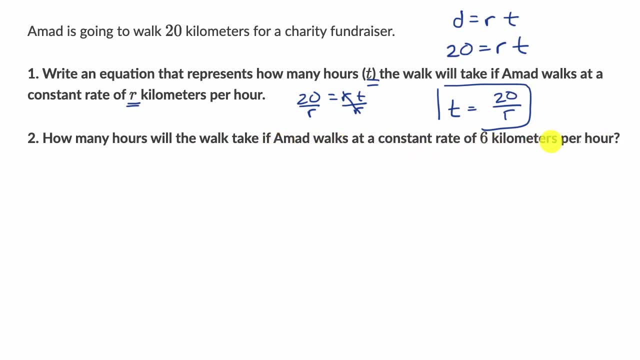 if Ahmad walks at a constant rate of six kilometers per hour? Well, here's an example of that, where they are giving us the actual rate and they want the time. So we just take the six and replace it in for R, So we get: T is equal to 20 over six, which is 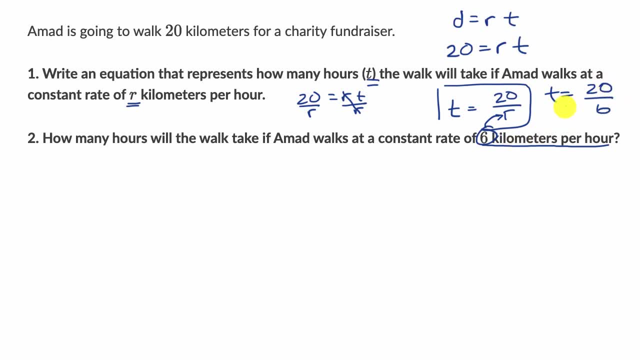 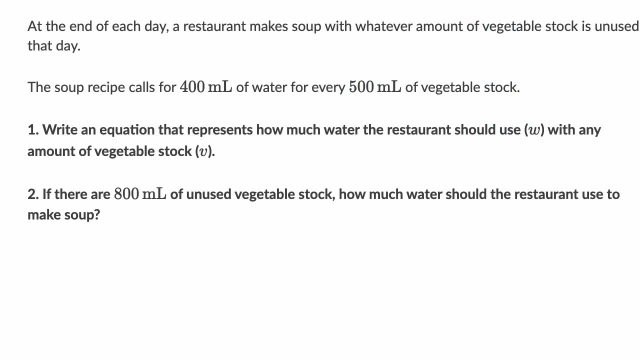 three and a third hours, which would be the same thing as three hours and 20 minutes, depending on how you wanna view it. Let's do another example here. So here we're told: at the end of each day, a restaurant makes soup with whatever amount. 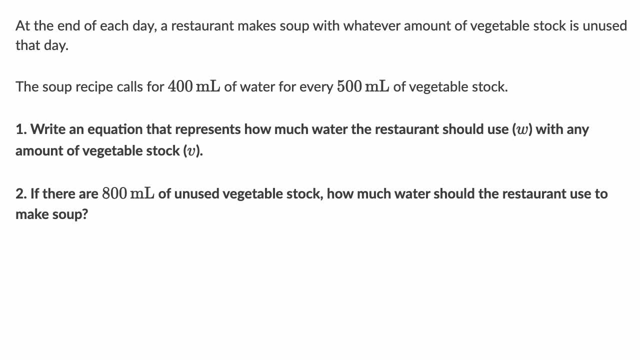 of vegetable stock is unused that day. Let me recenter this a little bit. The soup recipe calls for 400 milliliters of water. for every 500 milliliters of vegetable stock, Write an equation that represents how much water the restaurant should use. 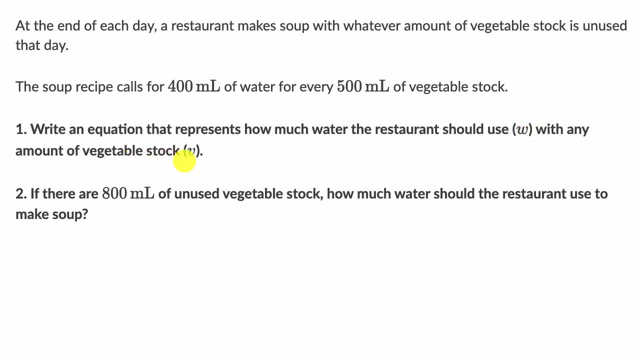 and we'll use the variable W with any amount of vegetable stock B, All right, and then we'll do part two right after that. So let's look at this: 400 milliliters of water for every 500 milliliters of vegetable stock. 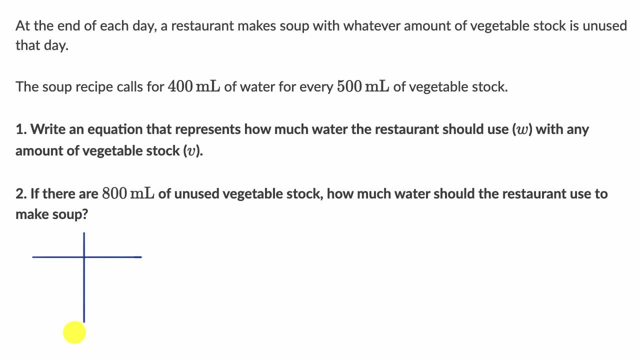 And so to get my head around this, I like just to think about. let's put a little table here, And so you could say amount of water. let me write it this way: water and vegetable stock, Vegetable stock. So for every 500 milliliters of vegetable stocks, 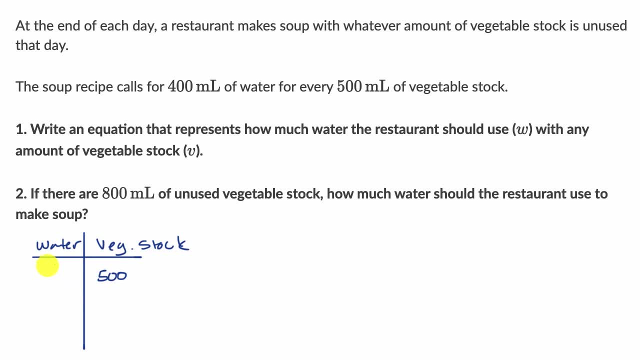 if you had 500 milliliters of vegetable stock- and I won't write the milliliters- then you're going to have 400 milliliters of water. If you had 1,000 here, which is two times that. 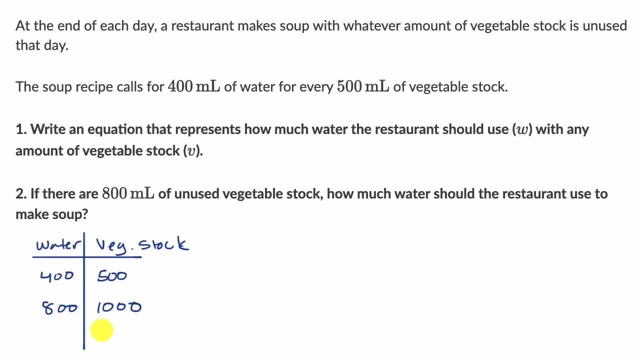 well, you're gonna have twice as much water, which is going to be 800. And so you can see this relationship that's forming, No matter what the vegetable stock is. if you essentially take four fifths of that, that is the amount of water. 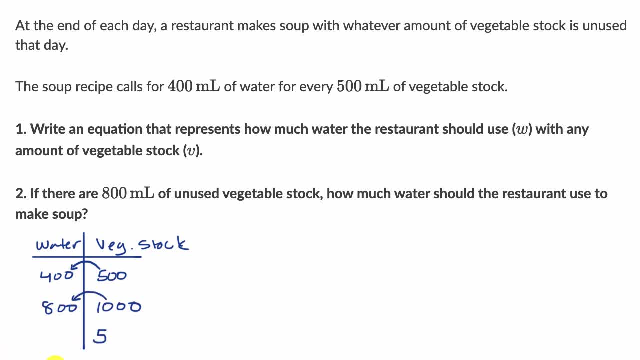 You take four fifths. that is the amount of water. So if you had only five milliliters of vegetable stock, you take four fifths, you get the amount of water. So another way to think about it is the water that you need to use is going to be four fifths. 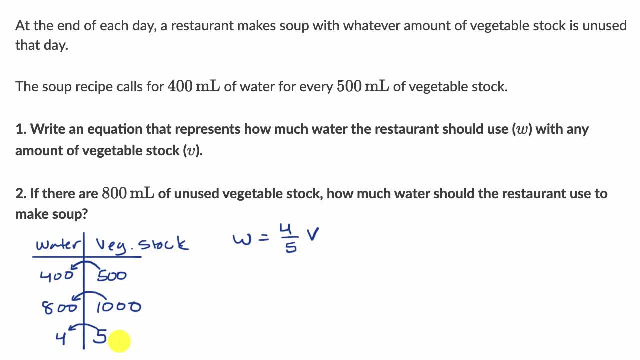 of the amount of vegetable stock that you are going to be using, And so, actually, we just did part one. We wrote an equation that represents how much water the restaurant should use with any amount of water, And so we're gonna take the amount of vegetable stock. 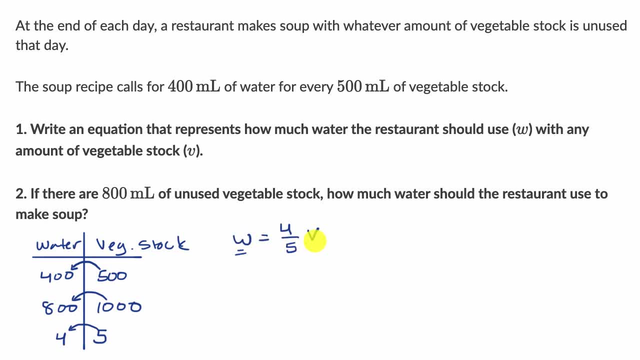 And the way that they phrased it. we're solving for W, given some V that you might have, And since we're solving for W here, we would consider W the dependent variable and V as the independent variable. You can give me different Vs.